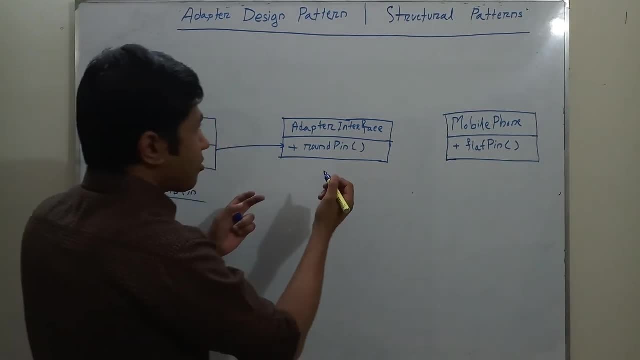 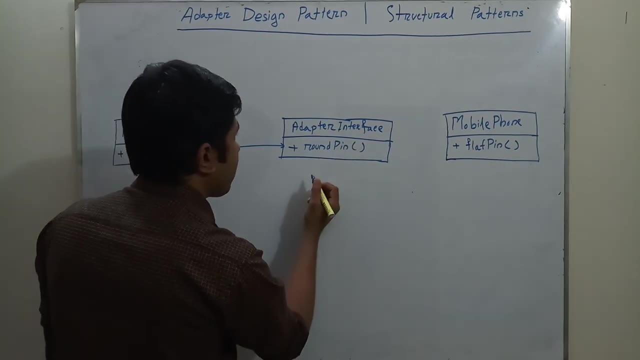 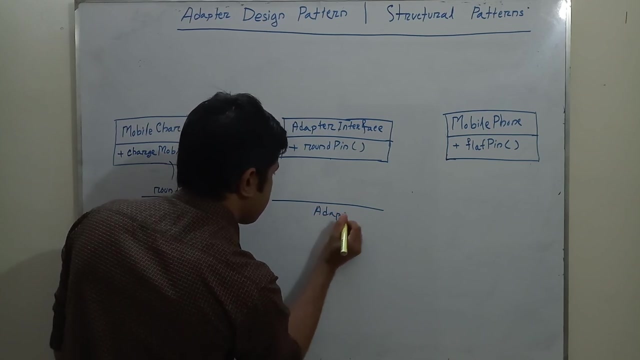 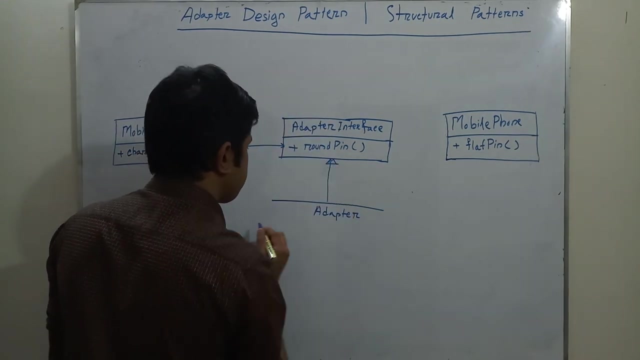 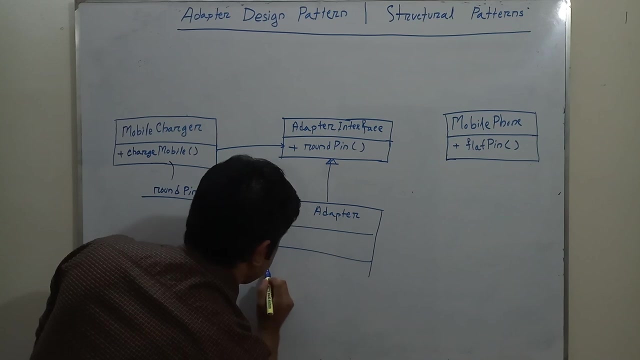 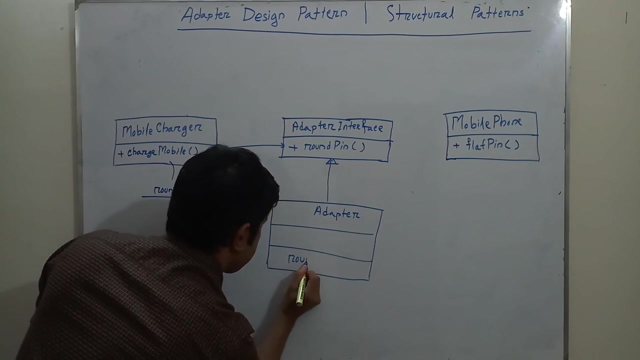 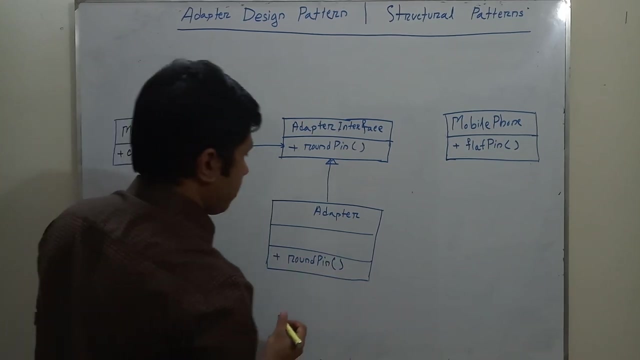 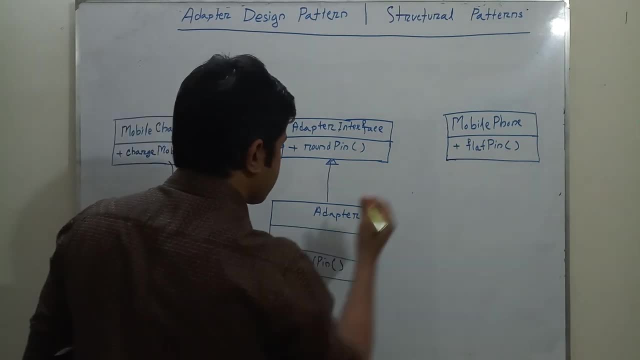 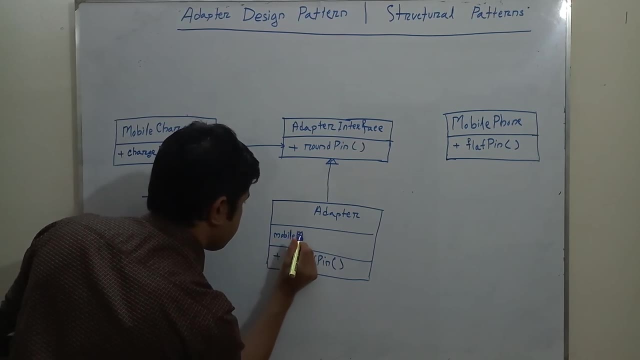 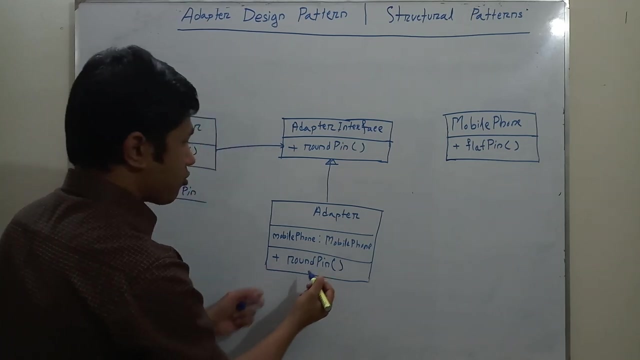 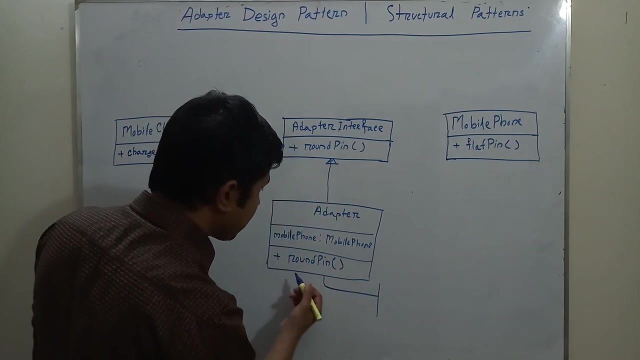 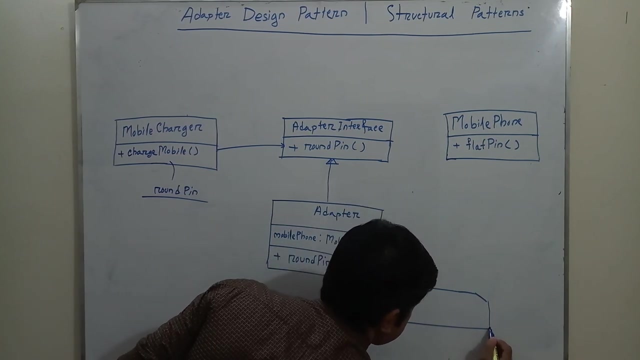 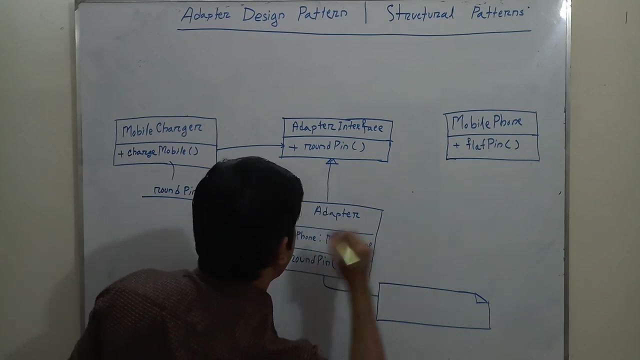 we need to access the mobile phone, which is a flat pin. So first create an instance of the mobile phone And in the function of round pin we will access the mobile pin. so the functionality of the round pin will be here. from round pin, we will access the flat pin here, the instance of the mobile phone. 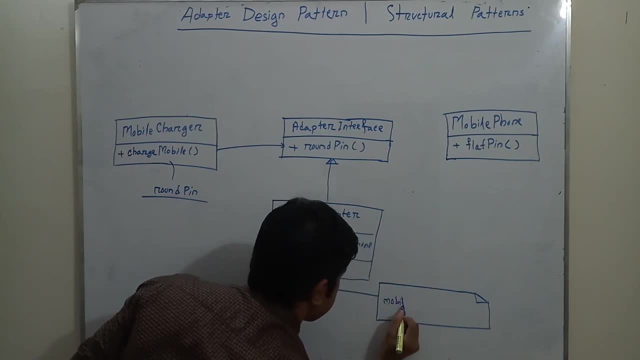 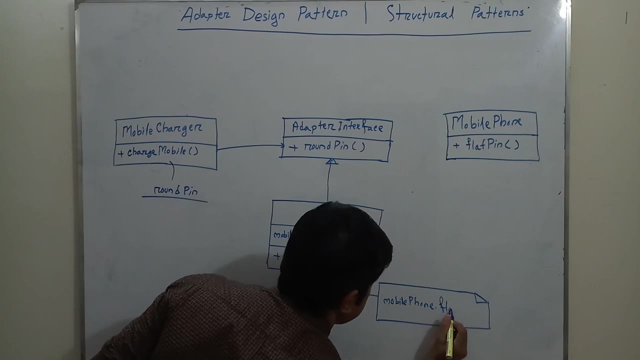 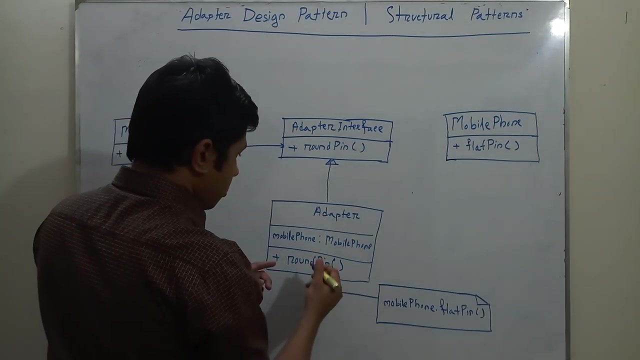 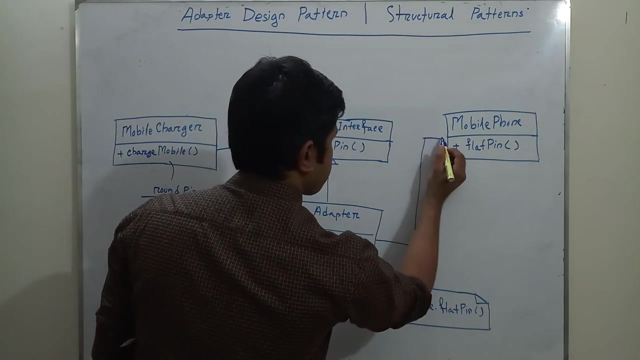 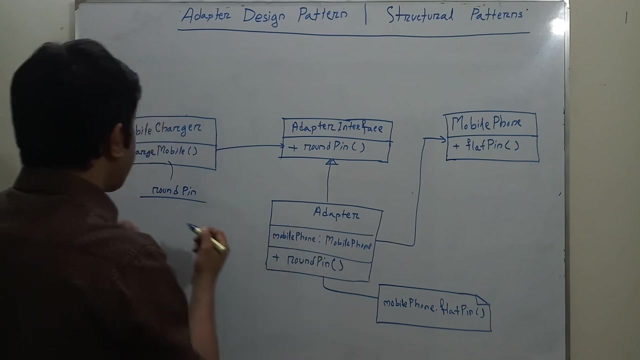 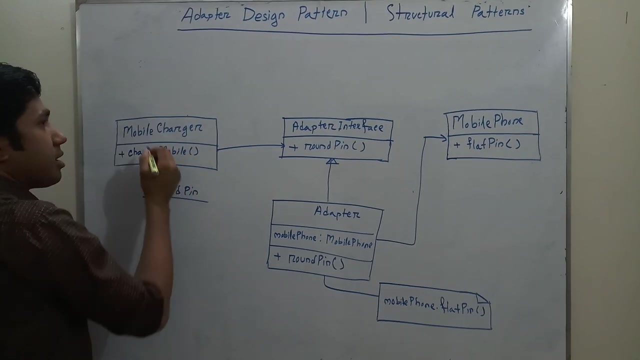 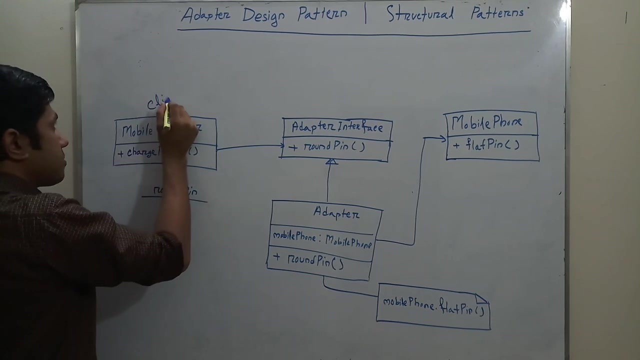 is mobile phone and we will access the flat pin. so the round pin function will access the flat pin function of the mobile phone here here, here. so now we can charge our mobile charger to charge the mobile phone through our adapter. so this is the client in adapter design pattern. the name of this part is client.